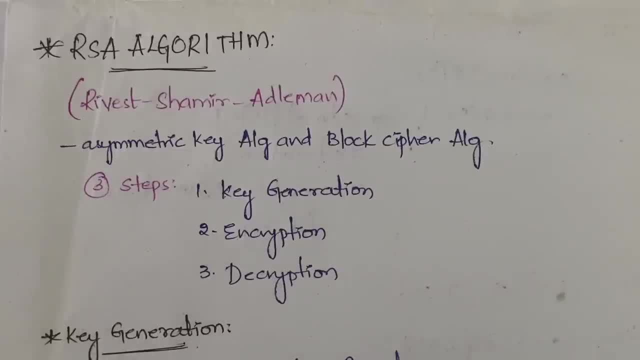 First of all, till now, we have learned some algorithms, like we have learned DES, AES, Blowfish and we have learned RC4 algorithm. So we have learned some symmetric key algorithms. But now from now, whatever we are going to learn, it may be RSA, it may be Algamal cryptography or Diffie-Hellman cryptography. 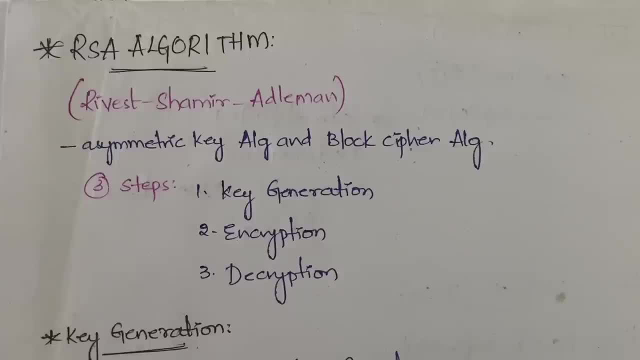 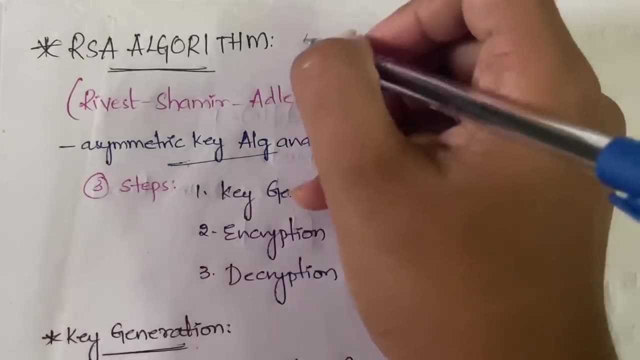 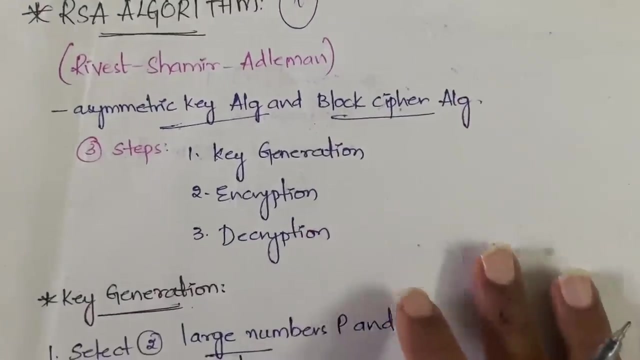 Knapsack algorithm we are going to learn. So all these will come under the asymmetric key cryptography algorithms. Okay, got it. The first one that we are going to learn is the RSA algorithm. So let us quickly- and this is a block cipher algorithm- Got it? So let us quickly go into the video. 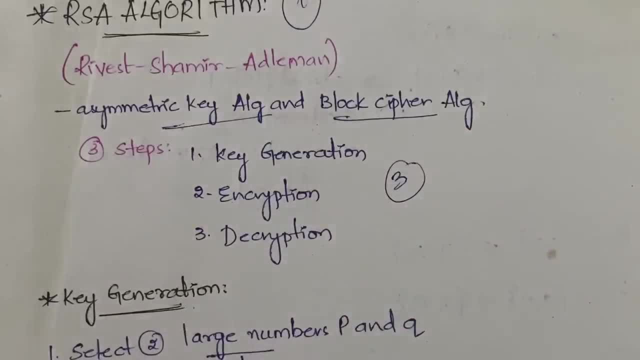 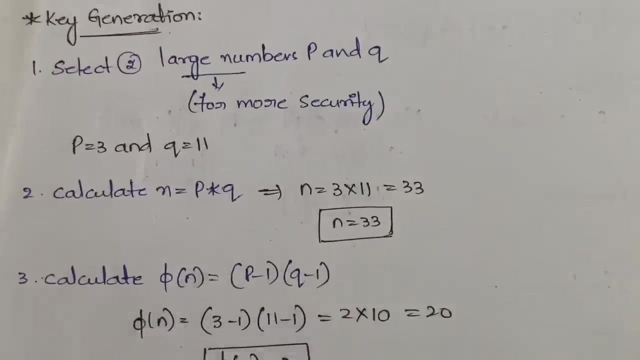 So here you have again three steps: common key generation, encryption, decryption. Okay so encryption, decryption will be very easy. Key generation is also, of course, easy, but it has some steps. It is somewhat lengthy, Okay. so first let us see the key generation process. First, what you have to do is I have- I have written the steps and simultaneously example also done. 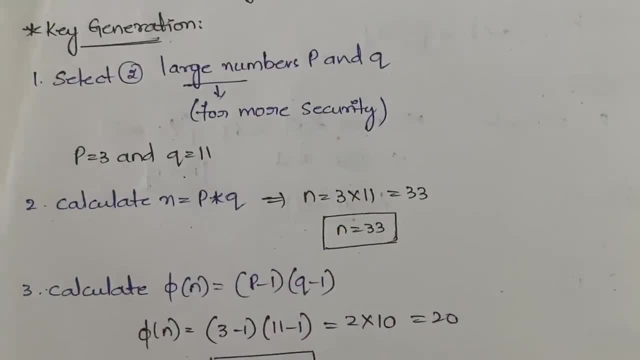 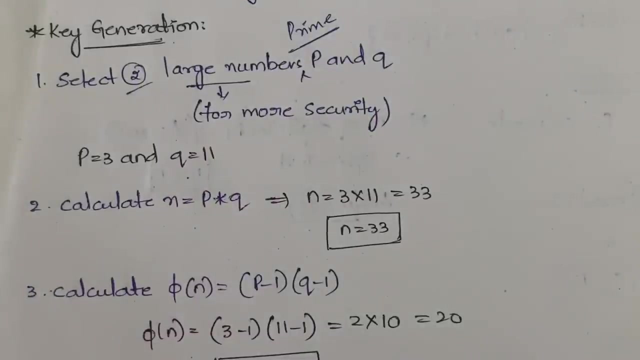 The steps are in blue color and the example is in black color, if you can see. So first, what you have to do is, in the first step, you need to select two large prime numbers: P and Q. Got it? So I think I forgot to write the word prime here. You need to select two large. Okay, leave it. I'm not sure whether it is prime or not. I'm sorry for that. Let us. I'll let you know by the end of the video. 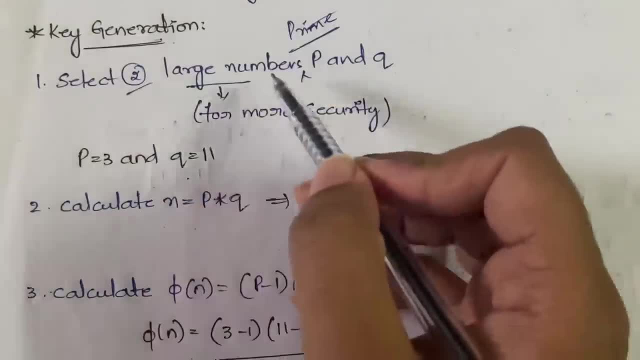 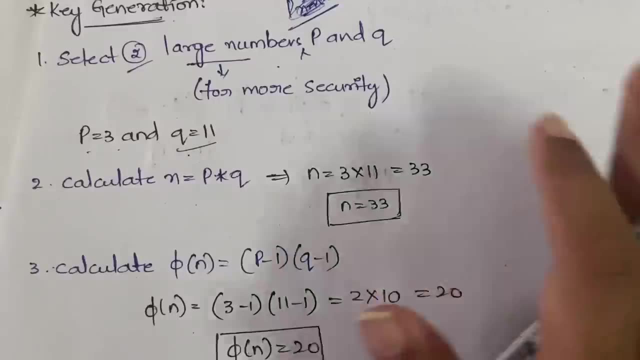 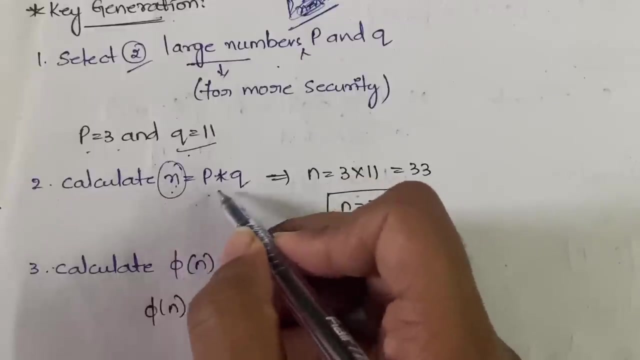 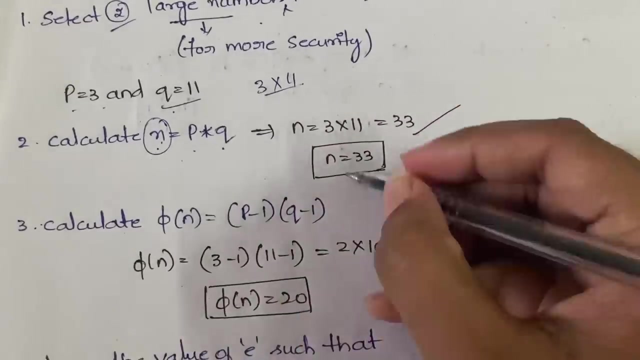 So you have to select two large numbers: P and Q. Why you have to select large numbers is for the purpose of security. Okay, so let us take P is equal to three and Q is equal to two. Okay, now, in the second step, what you have to do, you need to calculate the value of n. Okay, so what is the value of n is nothing but P into Q. So what does P here? three and what is Q here? 11. so three into 1133.. We got n is equal to 33.. Done. 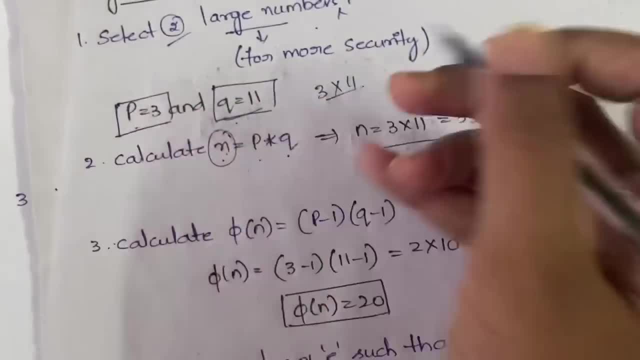 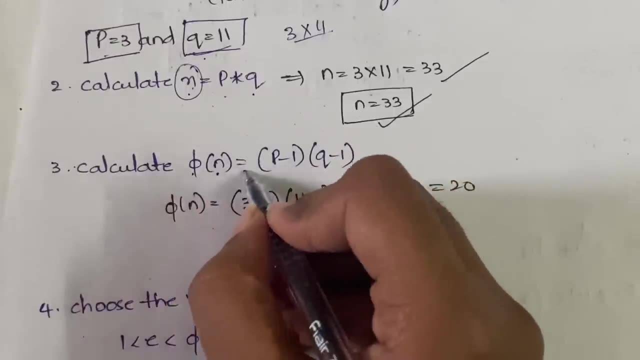 Right, So P is equal to three, Q is equal to 11 and n is equal to 33.. Next, in the third step, what you have to do is you need to calculate the value of five of n- five of n is equal to P minus one- into Q minus one. 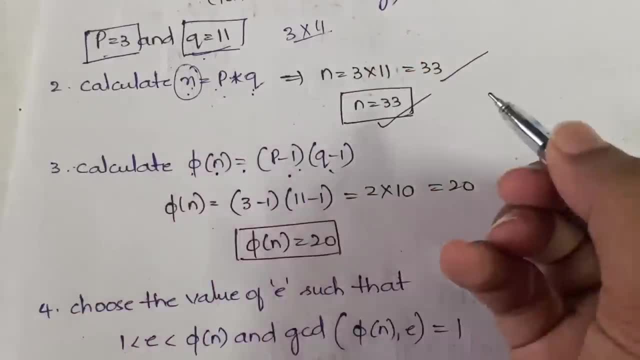 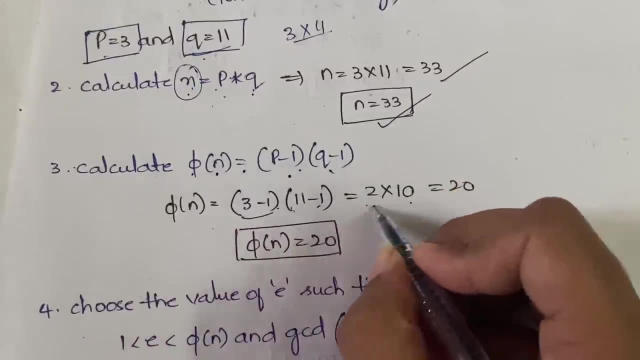 here you did directly p into q, red here p minus 1 into q minus 1. so what is p minus 1, 3 minus 1 into 11 minus 1. 3 minus 1 is 2 and 11 minus 1 is 10. so 2 into 10, you get 20 done. so 5 of n is: 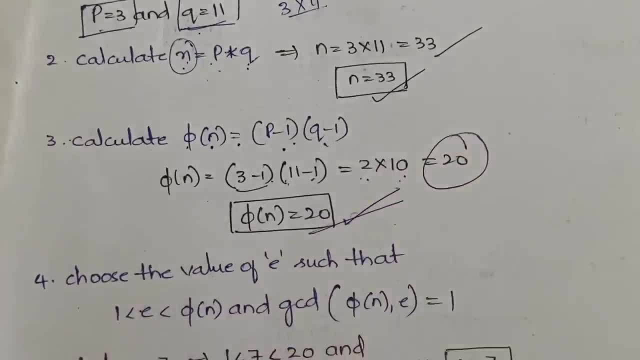 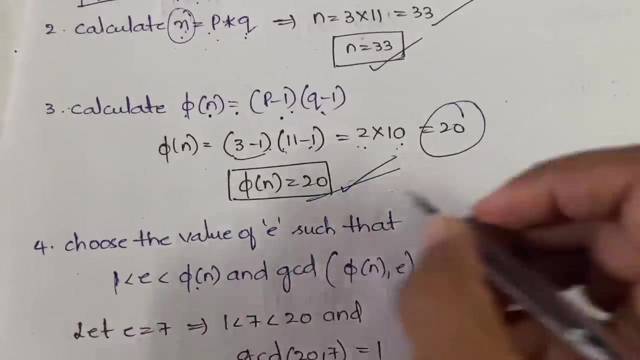 equal to 20. till here done clear. now you need to pick up the value of e. you need to choose the value for e. e stands for encryption, so you need to pick up the value for e so that the value of e should be between 1 and 5 of n. that is the value of e should be. for our example, it should: 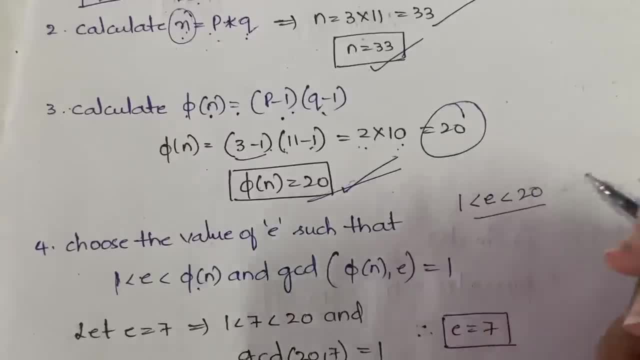 be 1 is less than e is less than 20, so you need to pick up a value between 1 and 5 of n. for our example, it means you need to pick up a value between 1 and 20, both exclusive right and also. 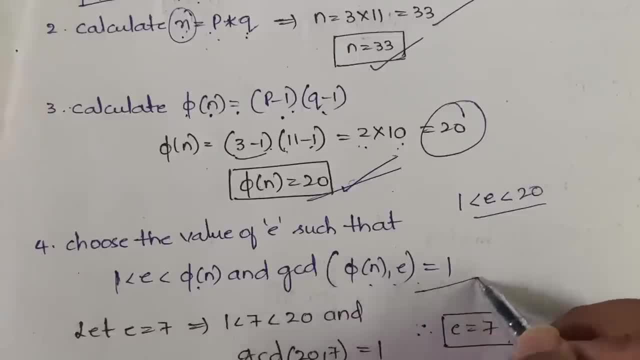 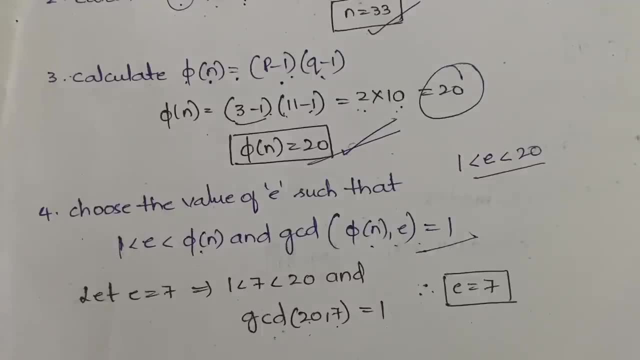 the gcd of 5 of n comma. he should be equal to 1. so the gcd of 5 of n comma e. so whatever e you're selecting, the gcd of that number and 5 of n, 5 of n, that is 20, has to be 1. so here, what is our 5 of n? it is 20, right? so the gcd of 20 comma, the. 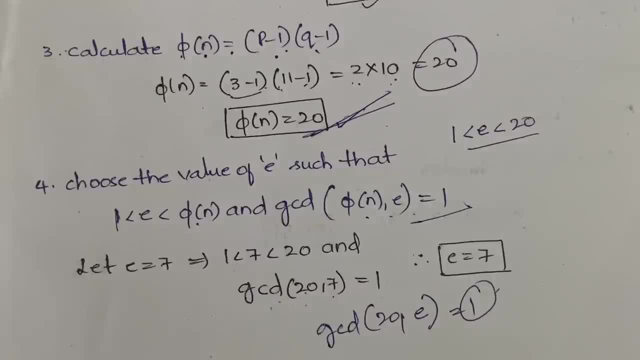 e should be equal to 1, so you can choose like 2, 2 and 20 gcd is not 1, 3 and 20 gcd is 1. so you can take 3, you can take. you cannot take 4, you cannot take 5, you can take 6, you can take 7. so we have 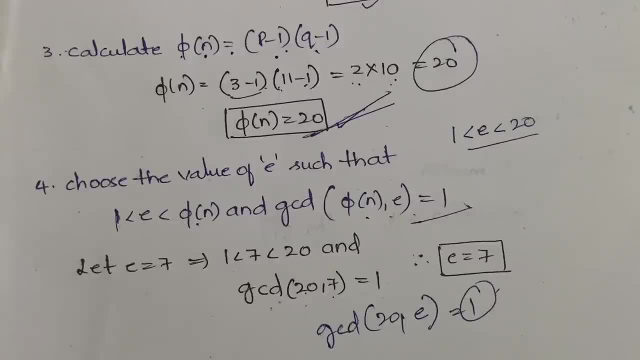 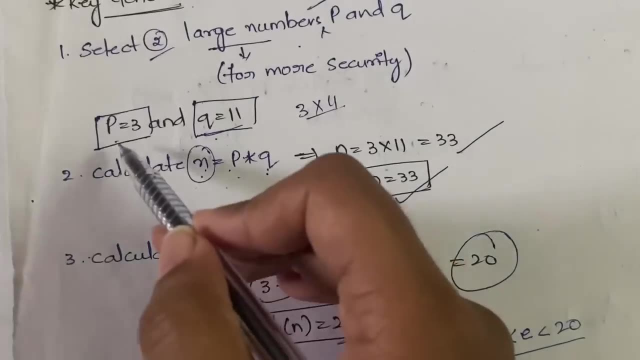 taken 7 here. let e is equal to 7. right, you can take anything. it's not like you have to take only 7. so we have taken here 7. got it now till now, what are the values we got? we got the value of p. 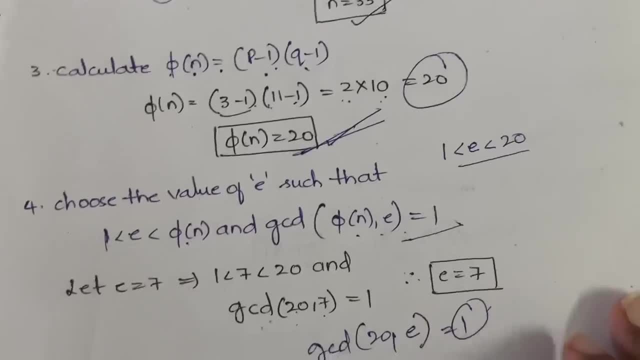 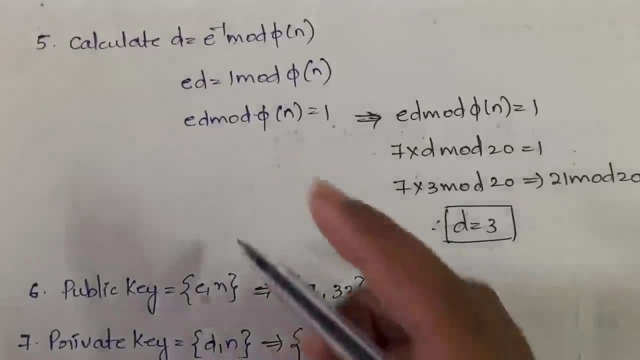 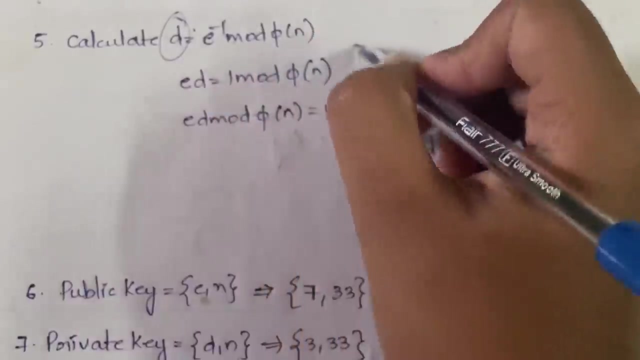 q, n, 5, 5 of n and e value. right now let us see the remaining steps. so the remaining steps follows like this: so first, what you have to do is you need to calculate the value of d. so for calculating the value of d, you need to do e power minus 1 mod 5 of n, but is. but this becomes a bit complicated. 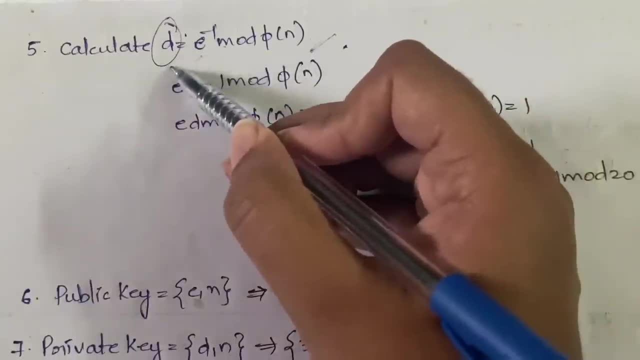 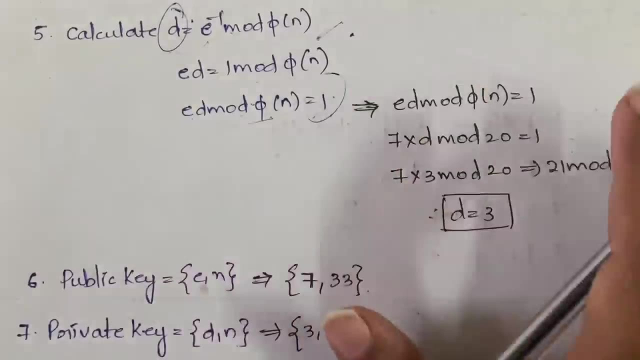 right. so let us make it easy. let us bring this e over. this right inverse becomes e. so ed is equal to 1 mod 5 of n. so ed is ed. mod 5 of n is equal to 1. you get okay. now what you have to do is you already know the value of e, you already know the value of phi. 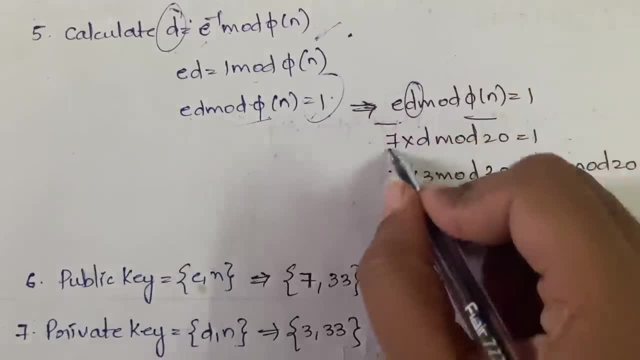 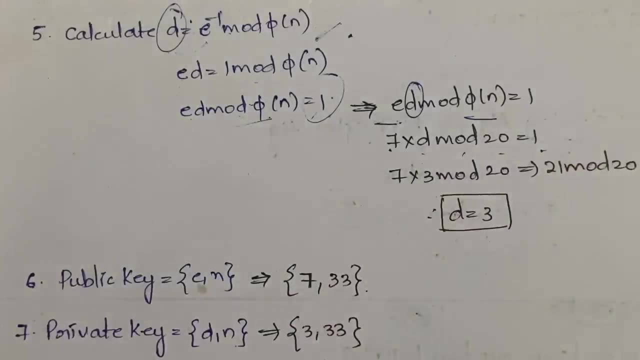 of n. you need to find out the value of d right. so 7 into d mod 20 is equal to 1 right. you need to check. 7 into mod 20: is it 1? no, it is 7. 7 into 2 mod 20: is it 1? no, it is 14 mod 20, so it is 14. 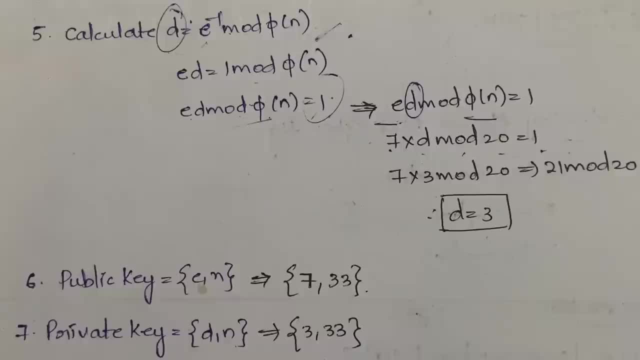 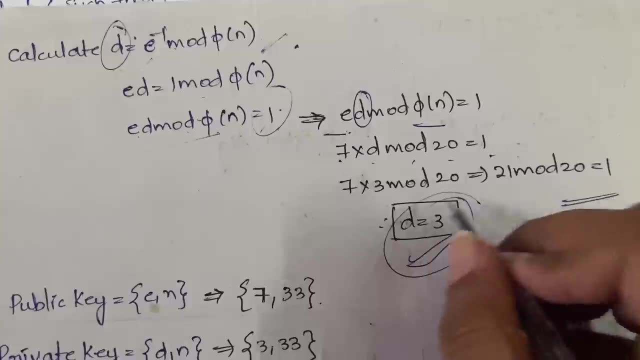 again 7 into 3 mod 20. 7 into 3 is 21, 21 mod 20. so the remainder is 1, so obviously 1. so you got 1 as the answer, right. so the value of d will be 3. you can fix it to 3. right now you have to generate. 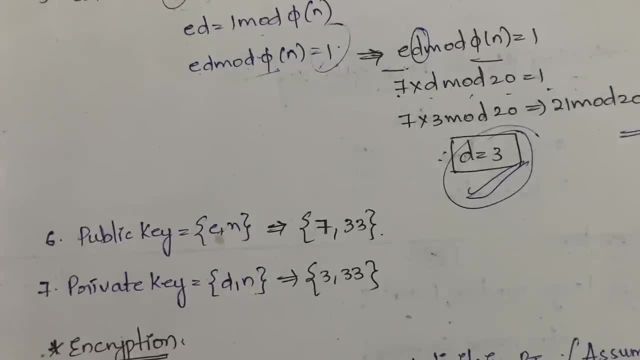 the public key and the private key. so in order to do the encryption or decryption, you need the keys right, you need both public key and private key, since it is an asymmetrical key- cryptography. so now you have to find out what is private key and what is public key. so for public key, it is e comma. 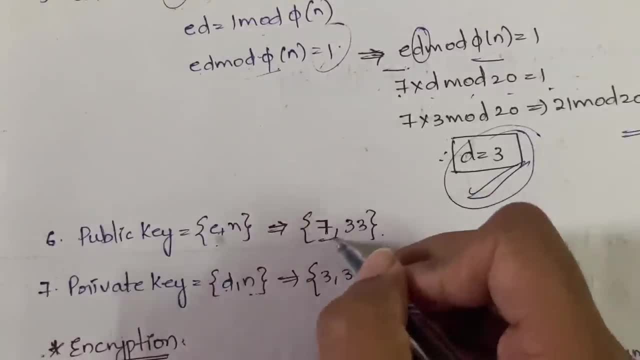 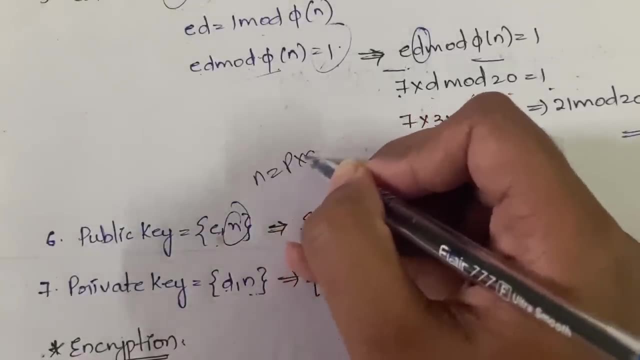 n and for private key it is d comma n. the value of e is 7. we already got it in the previous page right, and we already know the value of n as 33, because it is n is equal to p into q, 3 into 11. so 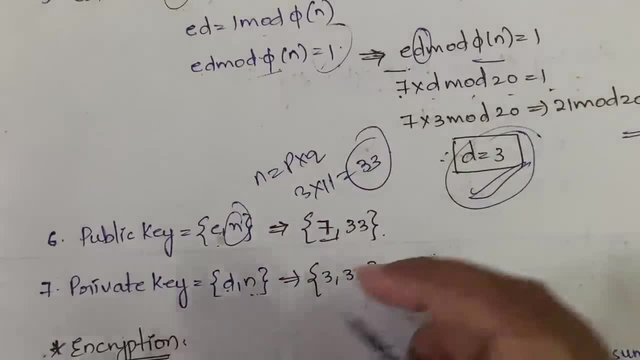 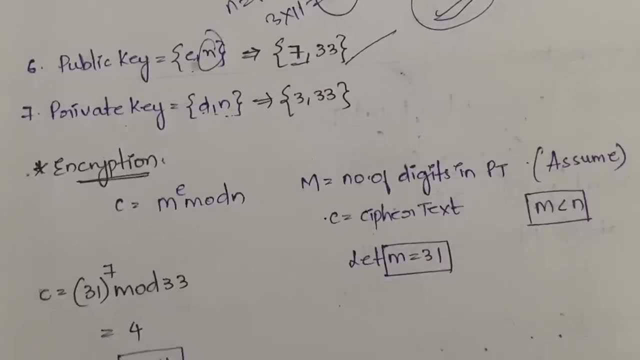 it is 33. we already know this done. perfect. so 7 comma 33 and private key is d comma and d just we got just now. so 3 comma 33 done. so we got the private key as well. now let us do the encryption and decryption. okay, so for encryption, what you have to do first is the formula for encryption. 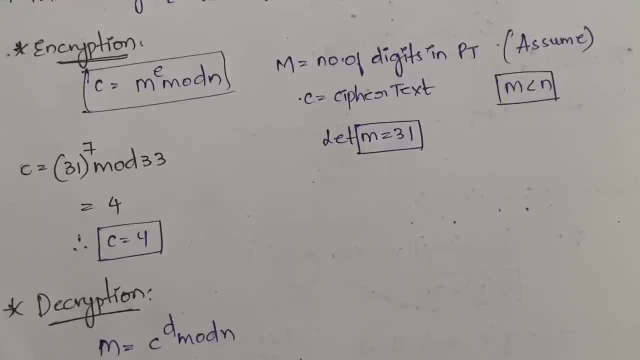 is this: c is equal to m power, e mod n. here you know what is e, you know what is n, and c stands for cipher text, okay, and m stands for plain text, got it. you don't know the value of m, but right, so you need to again assume the value of m. how? 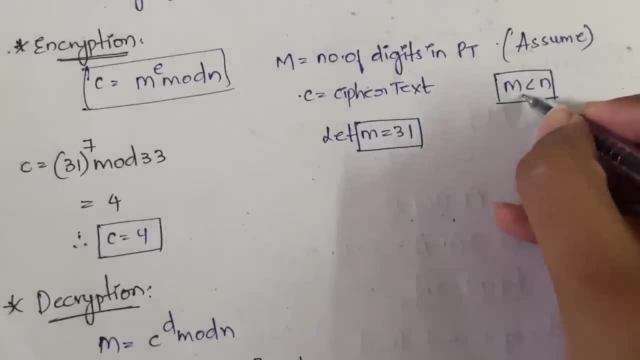 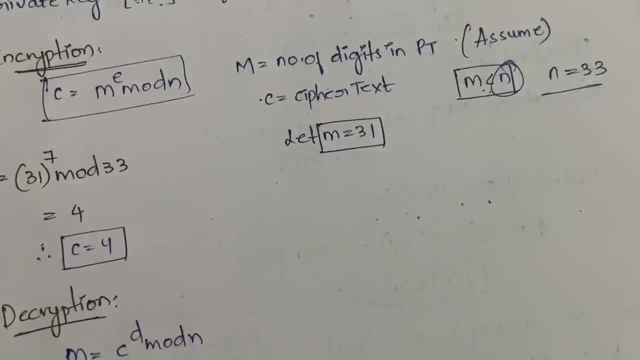 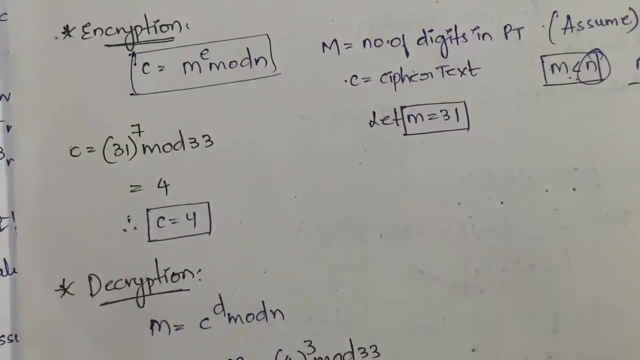 you will assume the value of m is m should be less than n. what is the value of n here? 33, right, so you can take anything which is less than 33. got it you need to assume. so we have taken 31 here. so 31 power 7 mod 33 is equal to 4.. so you can do it in the calculator, since calculator is a lot of. 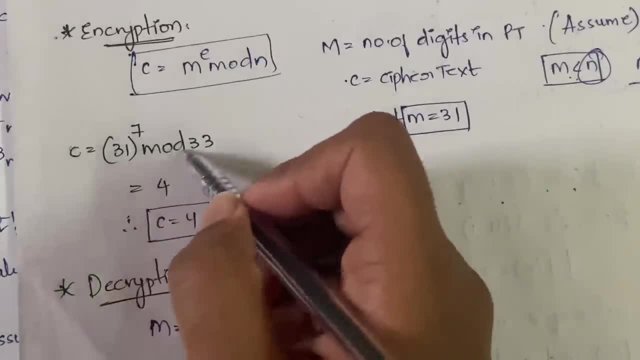 to the exam. you can take that and you can do this calculation. it's 31 power 7 mod 33. you will be doing so because you know e is 7 and n is 33. you already know. so you'll be getting c as 4.. 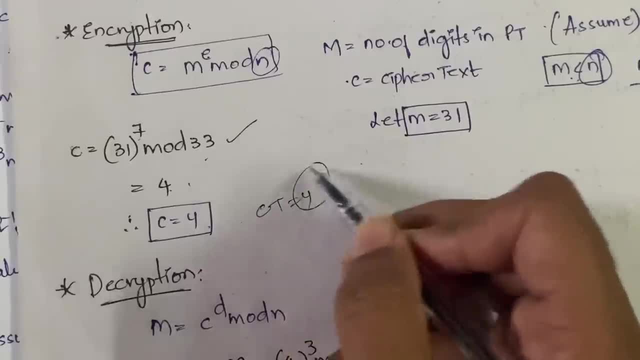 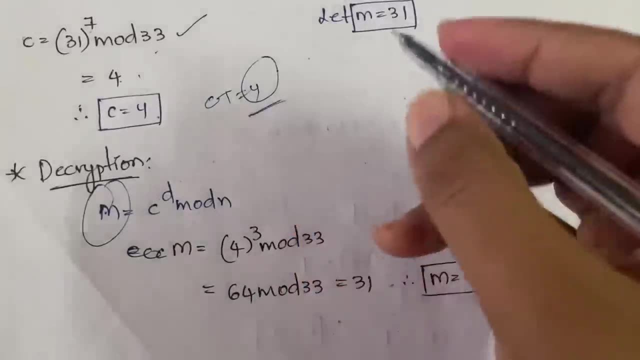 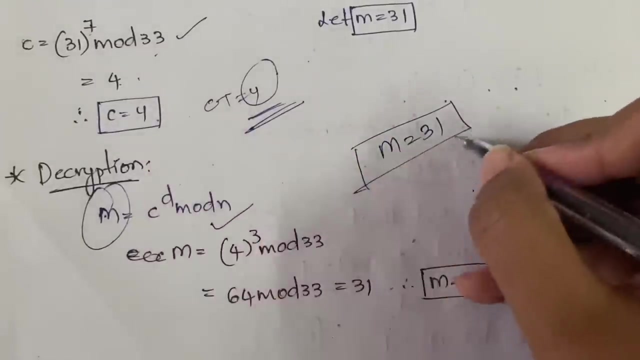 got it. so now our cipher text. we got it as 4. now let us do the decryption. in decryption process. what we will do, we will find out the value of m using this 4, actually what we have assumed the value of m as 31, right, so now, using this 4, you need to substitute in this formula: and if you, get the value of m as 31, then it is the number of thirty bool解. we smoke around 31 as there are. call it 400 plus k simмет. romantic answer, verse 2: um, this is where the value of m as 34 when.